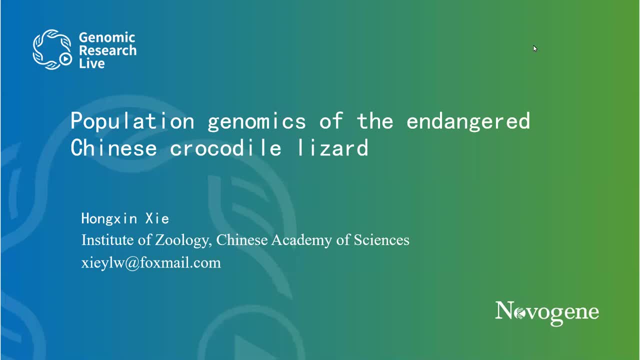 focusing on how genomic data helps to resolve the population history of Chinese crocodile lizards and provides insights into how genetic purging works in small wild populations. If you have any questions during the talk and would like to get an answer from the speaker, please leave your questions in the Q&A box. We will have some to discuss with Dr Xie after his. 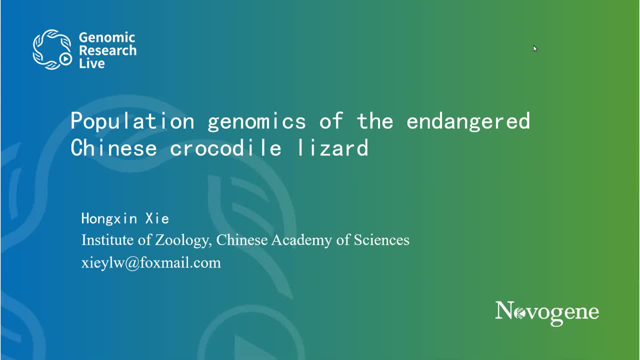 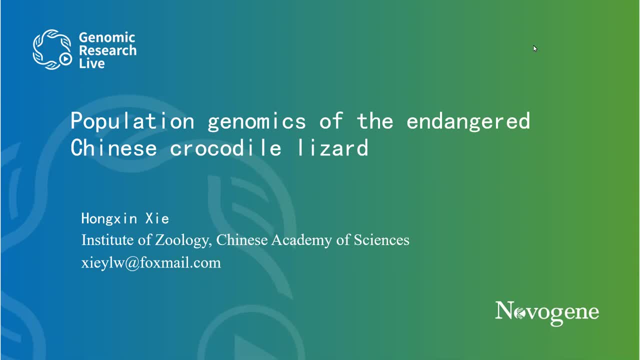 Dr Xie, please, Dr Xie, please, Dr Xie, please. Thanks for the introduction. I am very pleased to talk about our recent work on population genomics of crocodile lizards. Now shall we begin. 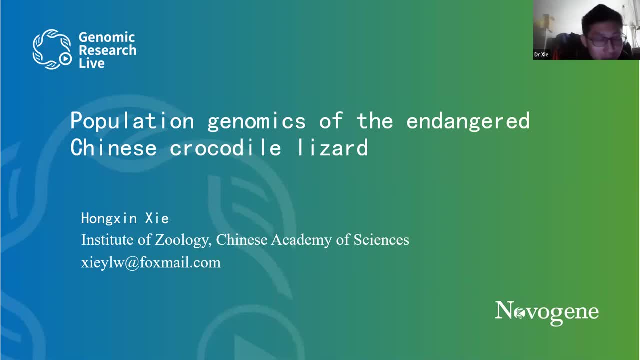 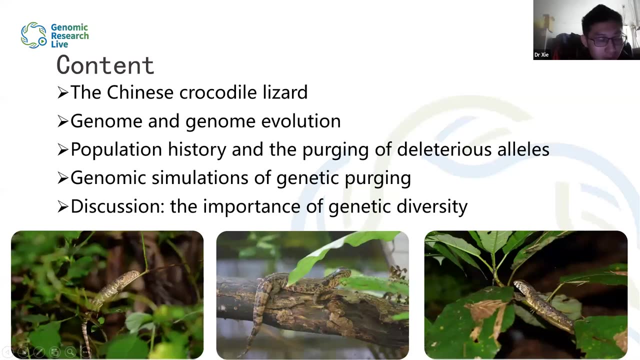 The main contents I want to share today include a brief introduction about focal species, the Chinese crocodile lizard, and then the leveraged genome we assembled, and then the main contents of our published paper, which is about the population history of crocodile lizards. 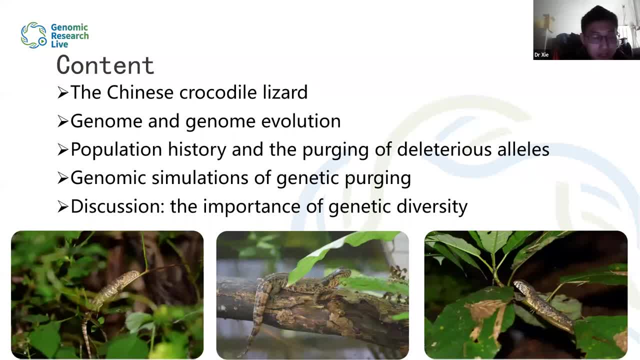 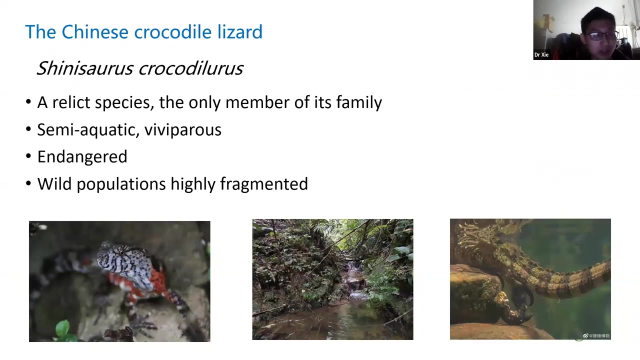 and the purging of deleterious alleles in its small populations. Finally, there is a brief discussion on the ongoing debate of the importance of genetic diversity and maybe some hints for future research. The Chinese crocodile lizard is a unique reptile species. It is first described in 1930 and is the 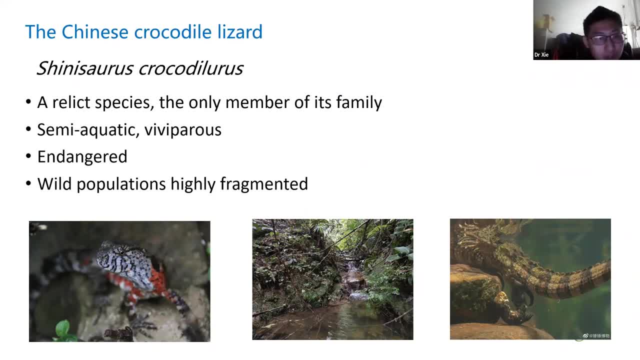 only member of its own family. The first photo here is a typical male crocodile lizard. The two most special features about it, in my own opinion, is that it's a semi-aquatic lizard- and baby parrots. The second picture is a habitat of crocodile lizards. 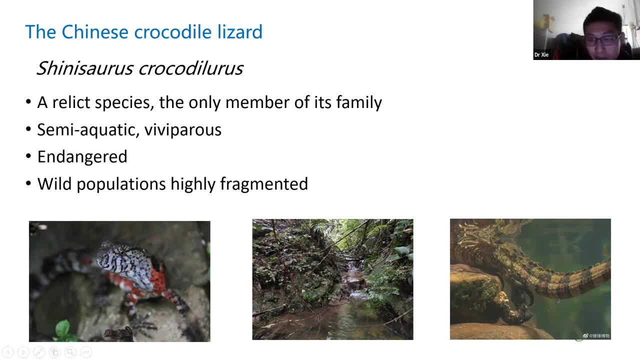 And the third picture is a female crocodile lizard giving birth to a baby lizard in water. The crocodile lizard is somewhat popular in the pet market, and so poaching and habitat destruction has already driven it to the age of extinction. Its current oil populations are small and fragmented. 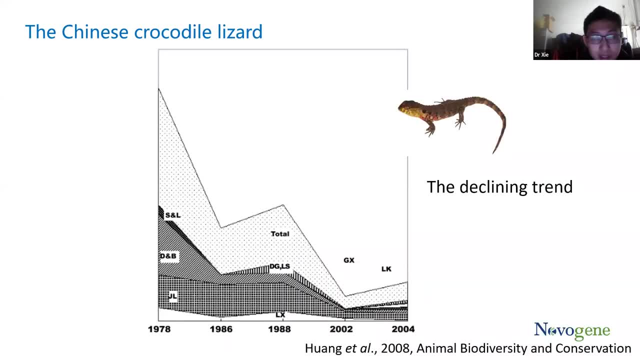 You can see that many studies have shown that the population of crocodile lizards are declining. New oil populations have been found in recent years, but the overall trend of its population is still not increasing but rather declining. Currently, there are about 1,000 individuals in the wild, or maybe less. 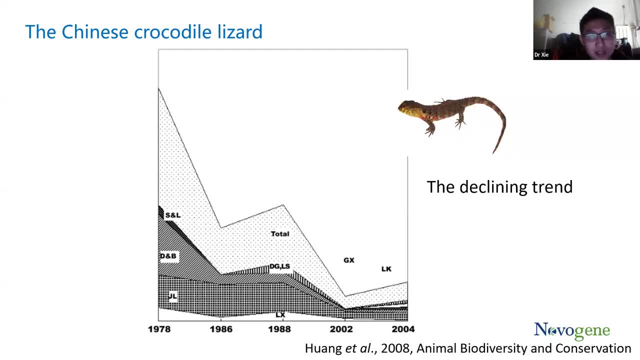 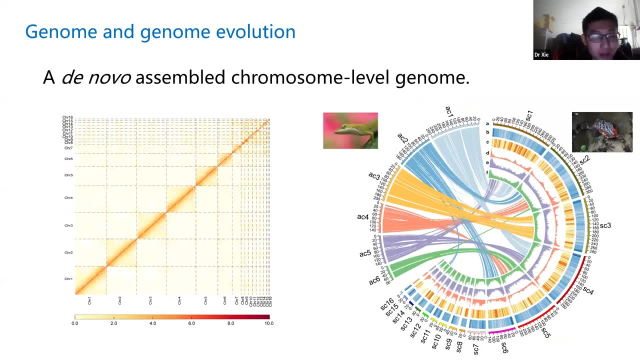 So, due to its characteristics and endangered status, a reference genome will be valuable for research on crocodile lizards. Now we assembled a crocodile lizard genome using PEGbio long reads and assigned the context to chromosomes using Hi-C data. 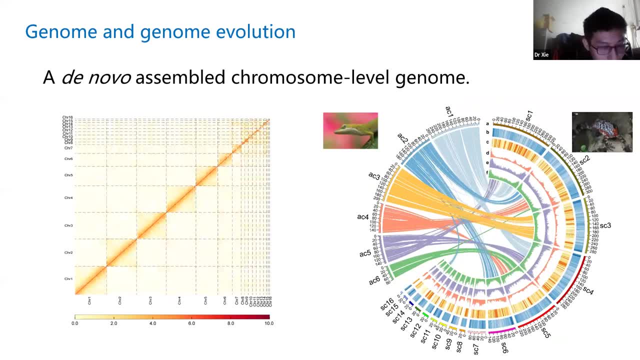 The left figure is the Hi-C interrectome plot of crocodile lizard chromosomes And on the right is a chromosome feature of crocodile lizard and synteny analysis between green-annealed lizard and male crocodile lizard. We can see that the chromosome is very large. 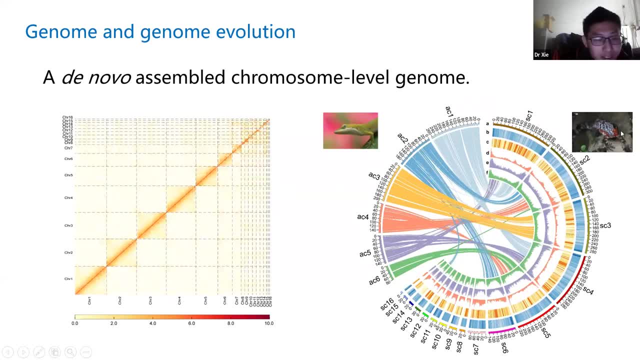 So this chromosome is very large. This chromosome is very large and the chromosome is very large. So we can see that the chromosome is very large and the chromosome is very large. So we can see that the chromosome is very large and the chromosome is very large. 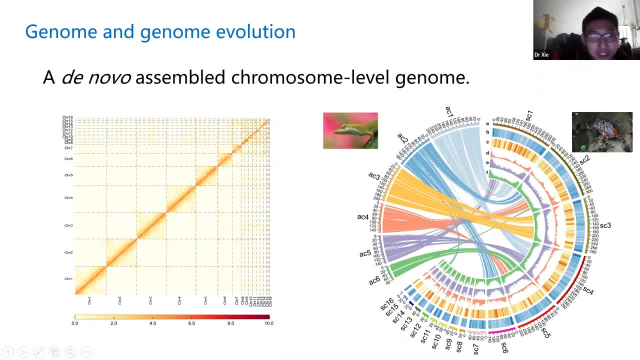 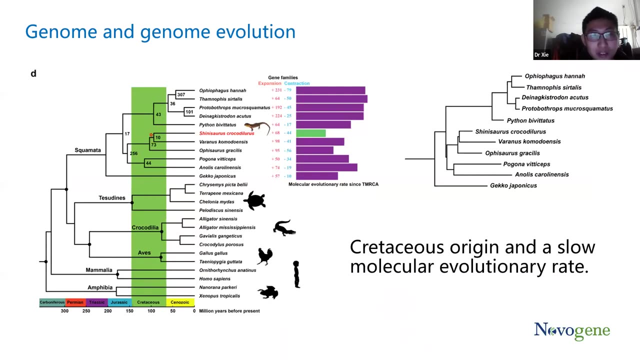 Actually, it does not give much information from this picture, but I just want to show that our genome is very good. We did some basic comparative analysis of crocodile lizard genome and other squamous species. For example, we found that the origin of crocodile lizards was dated back to 100 million years ago. 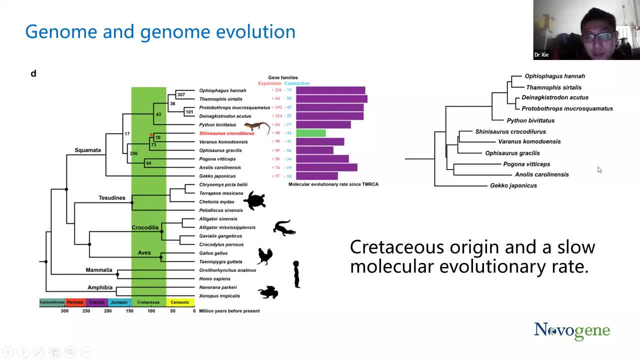 About in the period of Chretaceous period Is a time when dinosaurs was still on our planet, And we found that, compared to other lizards and snakes, the crocodile lizard has a relatively slower molecular evolutionary rate, which is consistent with this morphological primat Child. 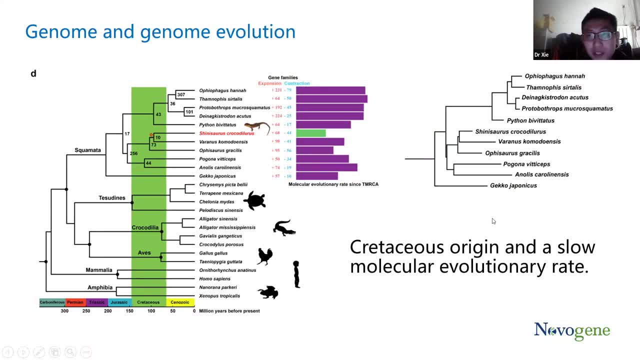 lizard is very ancient species. We found that is relatively slow. We also did some gene family analysis, the gene family evolution and positive static genes analysis. However, this is not the main points of our work, so we will just skip it today. 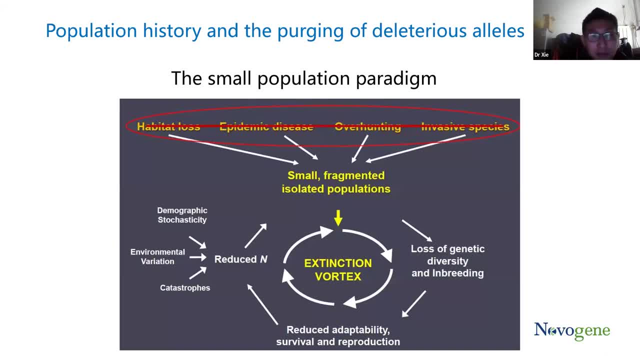 Now we come to the main part of our story. Here's some basic background information. In conservation biology, the small population paradigm is a very important research paradigm. It tells about a model that when a population has come to a small and fragmented may, due to many different kinds of reasons, 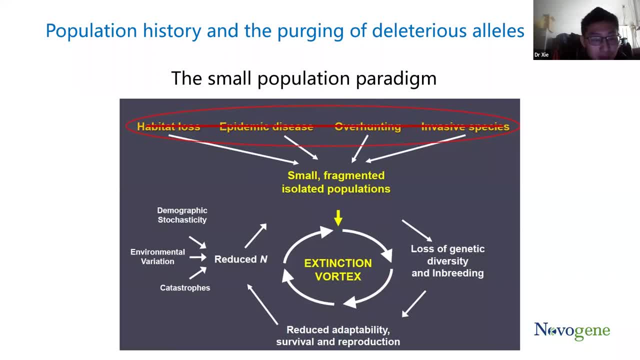 but when it's small. the loss of genetic diversity and increased stable of inbreeding will lead to the reduced fitness of the whole population, And then you are led to reduce the population size, and then reduce population size will again lead to reduced of genetic diversity. 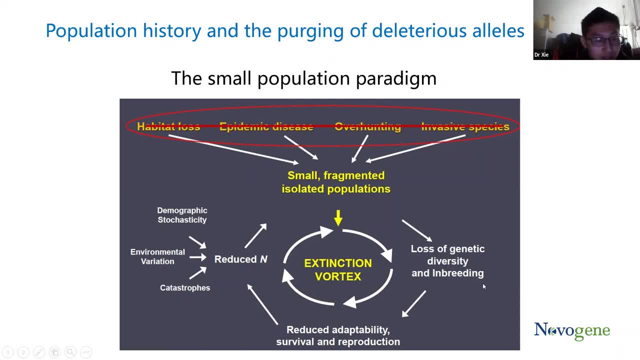 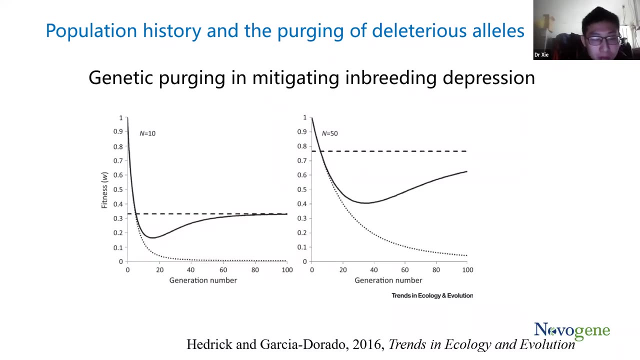 And this is finally led to extinction motifs, And this is a very well known model. However, The genetic purging of deleterious alleles may be able to mitigate inbreeding depression. The main evidences of genetic purging are in artificial populations. 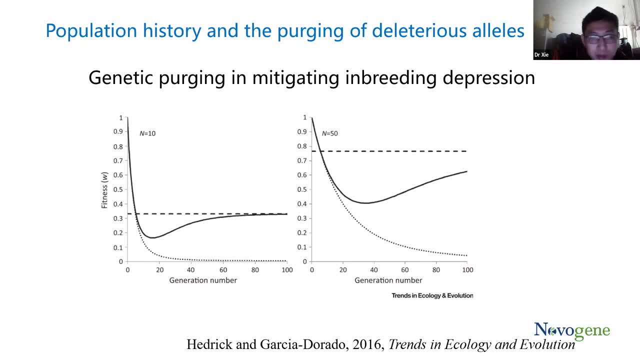 such in their populations or in breeding programs of animals or vegetables. It tells that the deleterious alleles are exposed to selection when inbreeding, And so it was purged from the population. However, in natural populations where the genetic purging works, 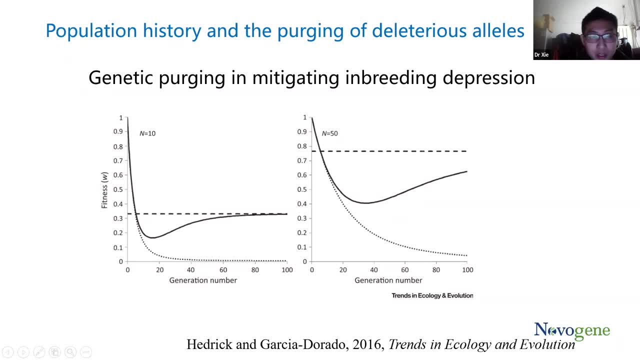 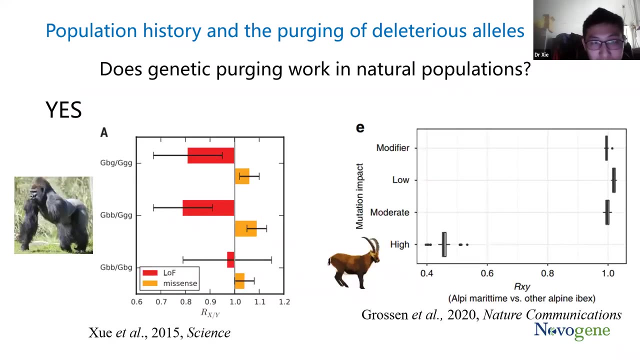 naturally in the wild is still conflicting. Recent progress in population genomics have revealed some facts, but the study results are somewhat conflicting. Let's see: Very typical research on the purging of deleterious alleles in the wild is one on modern gorillas. 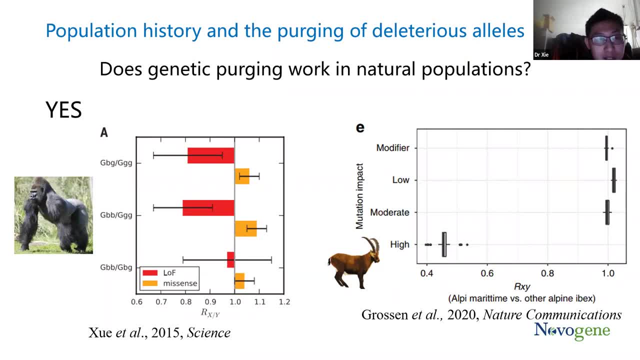 It uses a statistic which compares the modern gorillas deleterious alleles. there's L-OF function dose of function alleles to some populations with larger population size And I found that the L-OF mutations is relatively lower in the modern gorilla population. 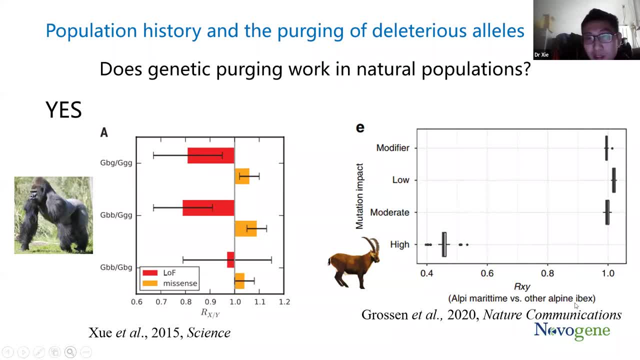 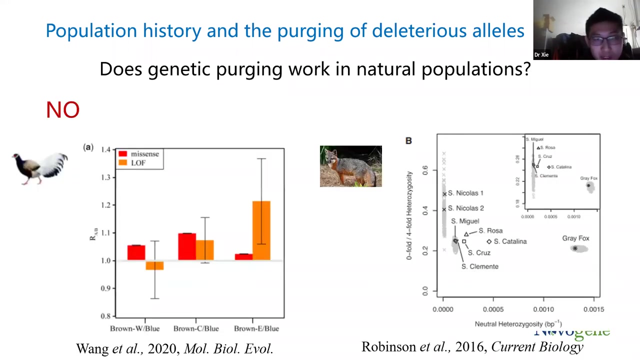 Another example is from the alpine ibex. It also uses the R-statistics And I found that the populations which underwent a severe bottlenecking have very significant lower L-OF mutations. However, there are other researches that have the opposite view, opposite results. 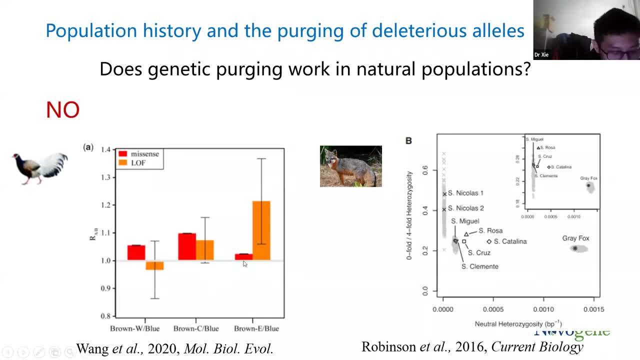 For example, in the study of this is: in the left is a brown-eared pheasant, a kind of chicken. It also uses the R-statistics And the results are opposite from the previous studies. The pheasant has a very low population size. 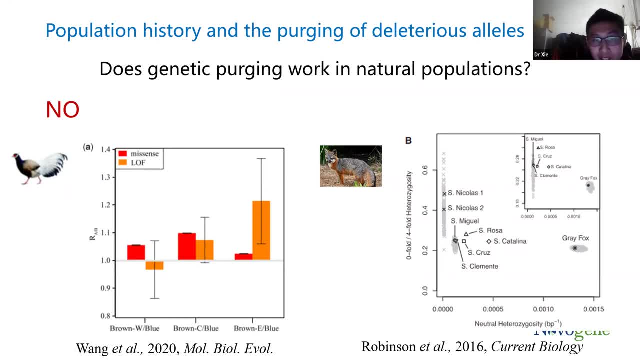 but its L-OF alleles in the wild. it's actually more than the larger populations In island force research. it uses another statistic, However. it also shows that the smaller population size- the population with smaller size, has larger- have larger deleterious alleles. 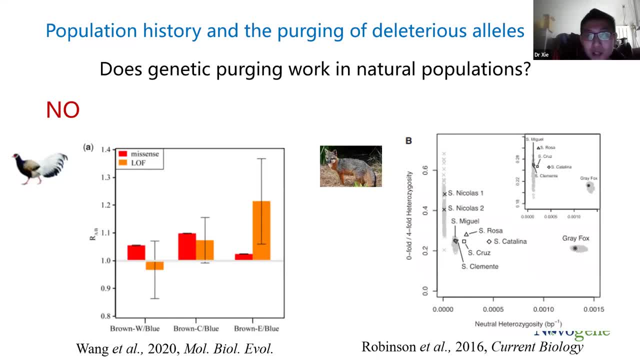 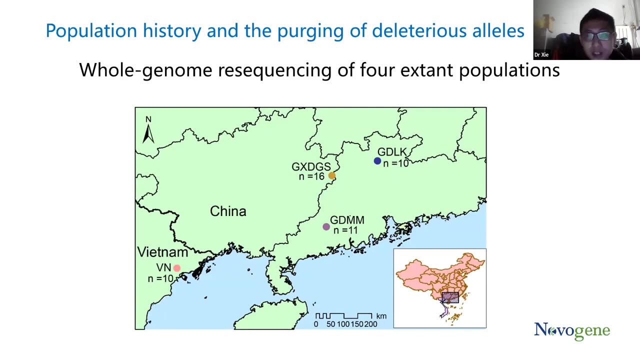 In this case, the problem of how pheasant really works in the wild and what's the pattern of it merits further research. So here we aim to use the the populations of crocodile lizards, and collect population-scale resequencing data. 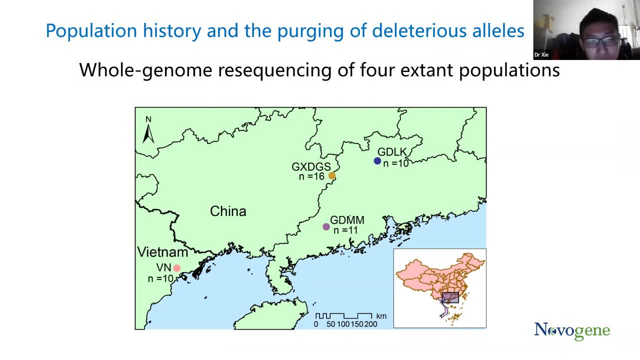 to solve this problem And this map shows the population, the samples we collect. We successfully collected four populations- This is, maybe, to our best effort, the only four exempt populations of Chinese crocodile lizards in the wild, And we collected a total of 47 individuals. 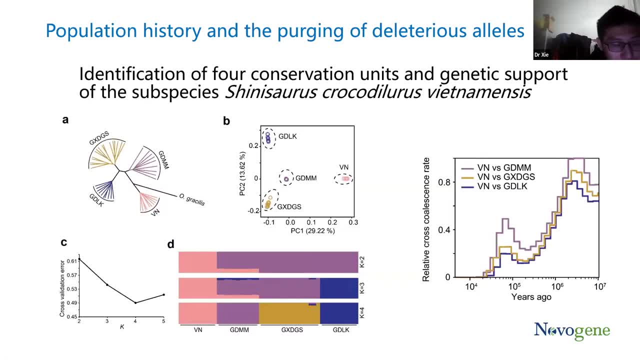 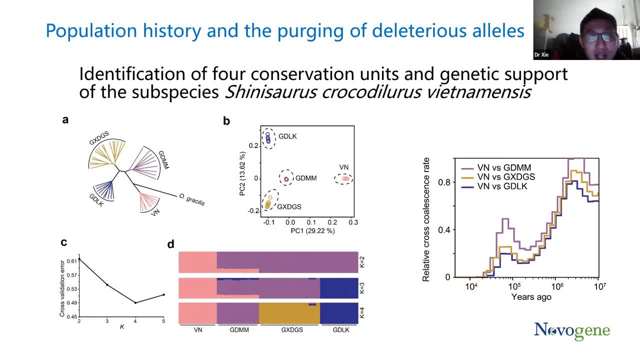 between these populations And is there any conservation units? We, from the results of the phylogenetic tree and the PCR analysis and the structural analysis from Adamistra, we confirmed that there exists four very genetically divergent populations of the Chinese crocodile lizards. 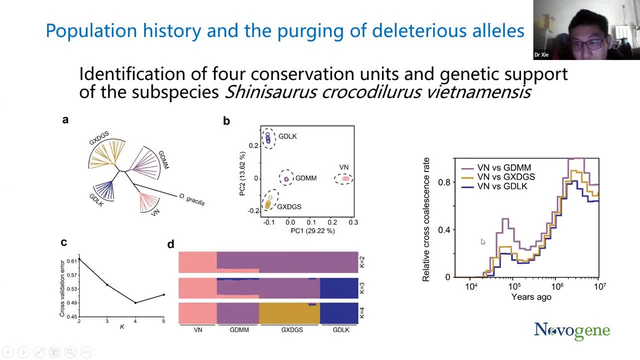 And we found that from the from the relative cross-correlation rate analysis in MSMC, we found that the Vietnamese, the VN population, the population from Vietnam is, have been fully diverged from the three Chinese populations about 20,000 years ago. 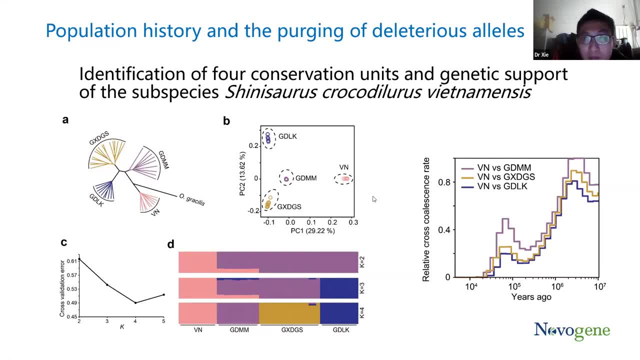 That's about in the last spatial maximum. So our results support a subspecies of Sunnysaurus chlordilis, the Vietnamese population subspecies of the Chinese crocodile lizards. And then to solve the population demography of the crocodile lizard. 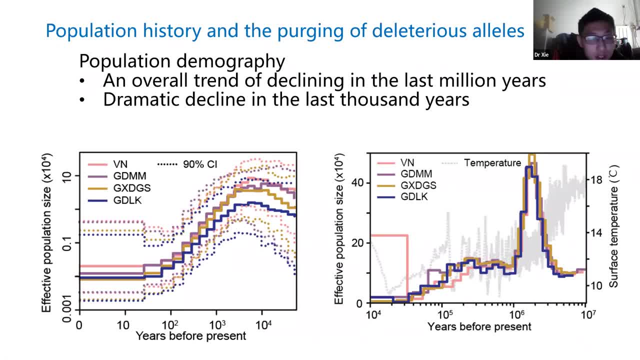 because we want to know its population history. So we use two methods to solve its population history. The one is a PSMC that is very popularly used. We solve its population history from millions of millions of years ago to about in the glacial maximum. 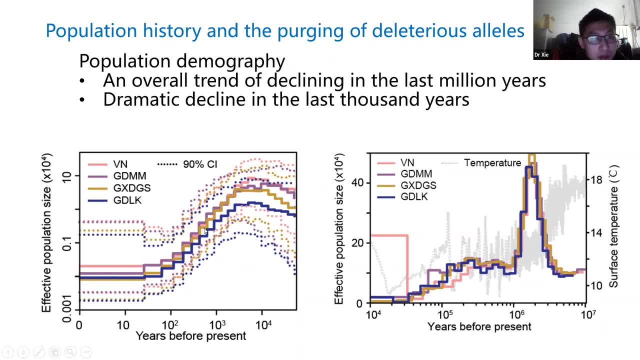 And the other one is a population size ABC. It solves about the population history about 20, 20,000 years ago to the present And we show that there's an overall trend of declining in the last million years of population population size. 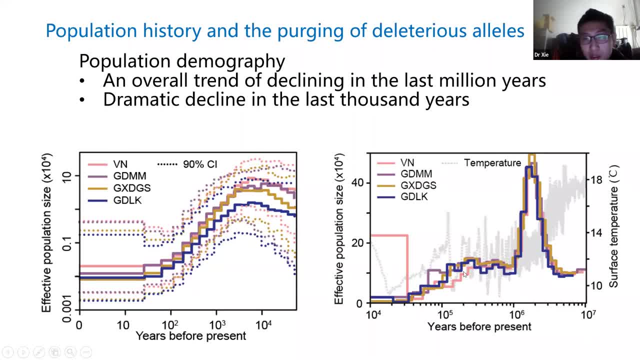 effective population size of a Chinese crocodile lizard. It's gradually declining, especially we see from last glacial cycle. there's a decline and a bottleneck in the last glacial maximum. Then the population expanded a little. but in the recent 1000 years 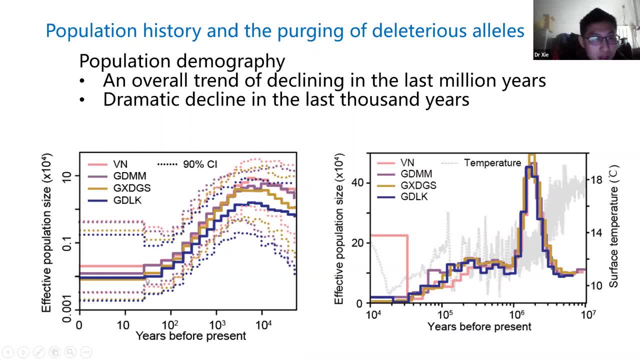 the population dramatically declined to a local minimum size in the recent years And maybe this is this describes the process of going endangered in the recent years. We also did a relation analysis To solve the individual relationships between our samples. We did this because we know the population size is small. 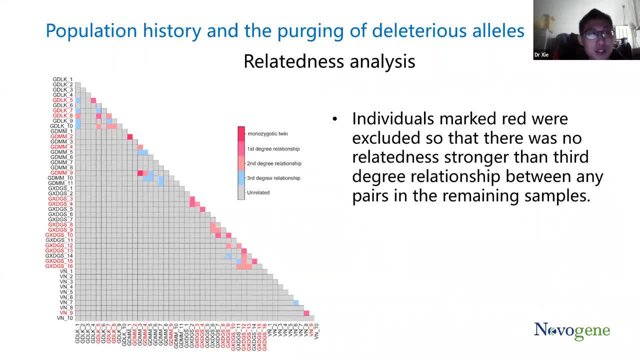 So it's very possible that we sample some individuals, but they are actually very close relationships, maybe siblings or parents and kids. So we need to do some statistical analysis in a foreign analysis. but these close relationships may bias our results, So we did a relation analysis. 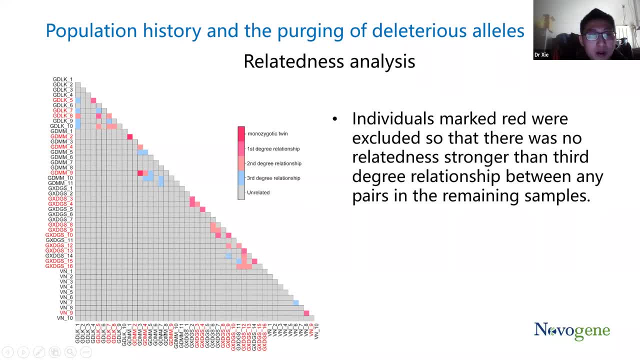 We did a relatedness analysis and excluded all the individuals that show possible close relationship. There's relationships stronger than third degree relationships And we and we excluded about 16 individuals And for all the other samples left, there's no close relationships between any pairs of the sample. 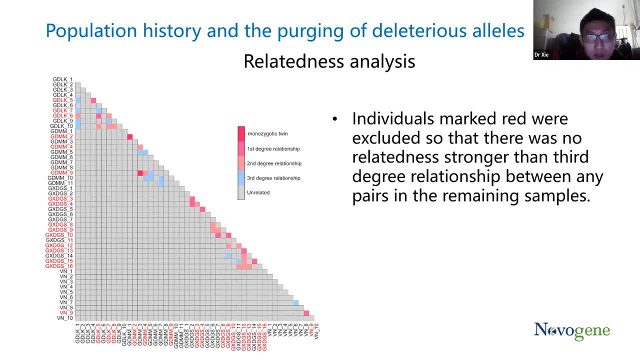 And based on this sample, we we analysis their genetic diversity and we did a relatedness analysis. And for all the other samples left, there's no close relationships between any pairs of the sample. So we did a relatedness analysis and excluded all the individuals that show possible close relationships between any pairs of the sample. And based on this sample, we also did a relatedness analysis And for all the other samples left, there's no close relationships between any pair of the sample And based on this sample, we we analyzed their genetic diversity and inbreeding level. 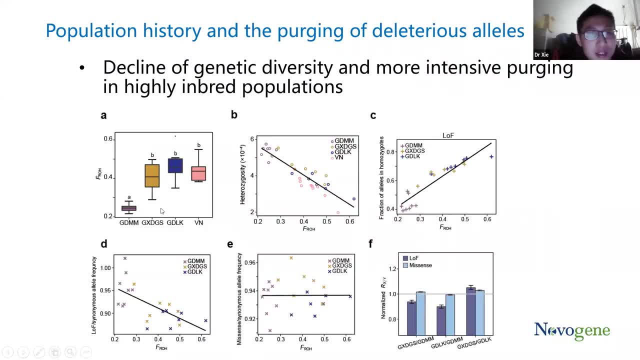 Firstly, we see a figure eight. FLH is a statistic that describes the inbreeding level of individual And we see from this product it is very obvious that the Guangdong bombing population is a population from China, is inbreeding level all FLH is significantly lower than other three populations. 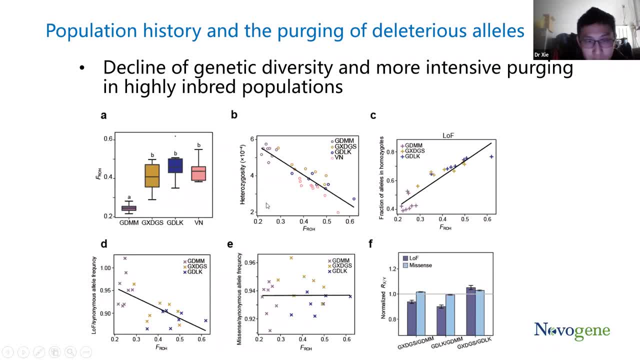 And then from figure three B we did a larger analysis, did the correlation between heterozygosity as a measure of genetic diversity of an individual, to the FRH. we show that the heterozygosity declines show a negative correlation with FRH. 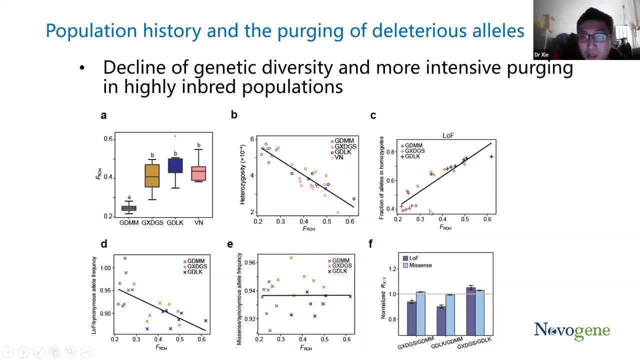 And we show that the fraction of alleles in homozygotes increases with FRH, which tells that inbreeding has already caused the declining of genetic diversity and overall genetic loss. But as the deleterious alleles are homozygotes in the inbreed population, then all changes have. 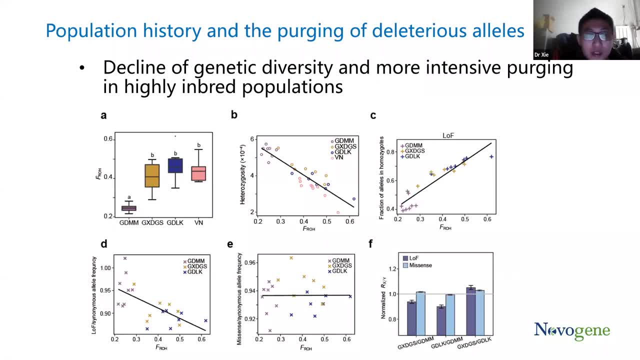 happened to its frequency. So we did another correlation with the frequency of deleterious alleles to its FRH and we found that it showed a declining trend. That means with more intensive inbreeding, the frequency of LOF alleles loss of function alleles seem to declining, which shows 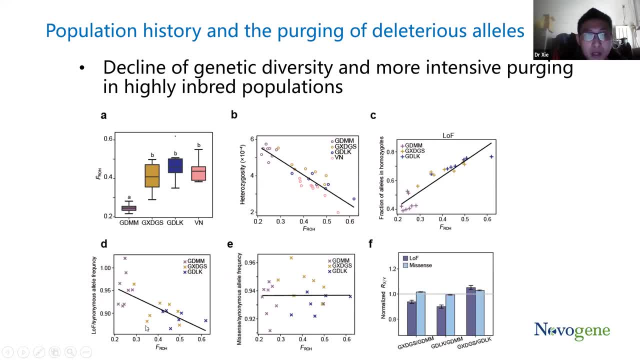 a trend signal of purging And if we see missense alleles, there's some alleles that are not that harmful to LOF alleles. The trend is there's no significant trend, no declining or not increasing. It shows that the purging was different in loss of function alleles and missense alleles. 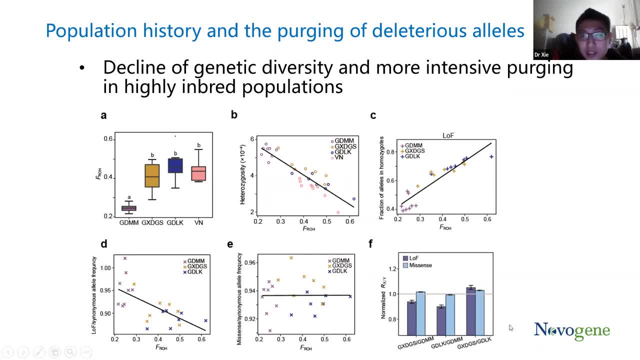 We use another popular R statistic. This statistic is to compare the differences of allele frequency between two populations. We found that compared to Guangdong-Mao Ming- that is the population with lower inbreeding level- the LOF allele frequency is lower in the more inbred Guangxi Da Guishan. 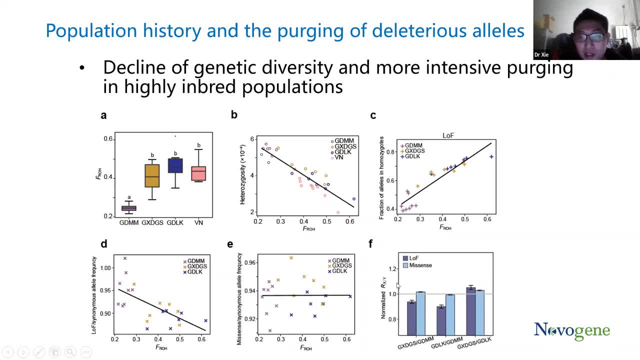 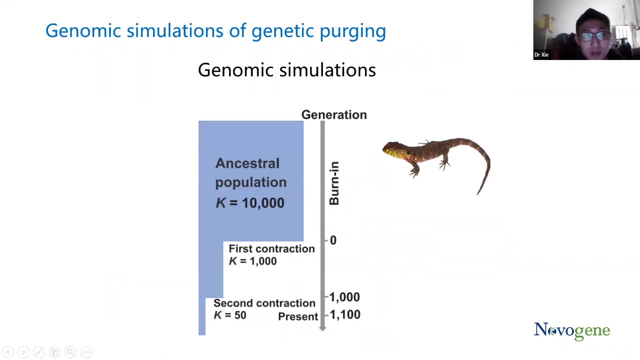 and Guangdong-Luokeng population, which means that the more inbred population has lower LOF mutation alleles. But for missense alleles the difference is not that big. This is consistent with the modern GARIA results. But then we want to see if the purging is really working in crocodile lizard populations. 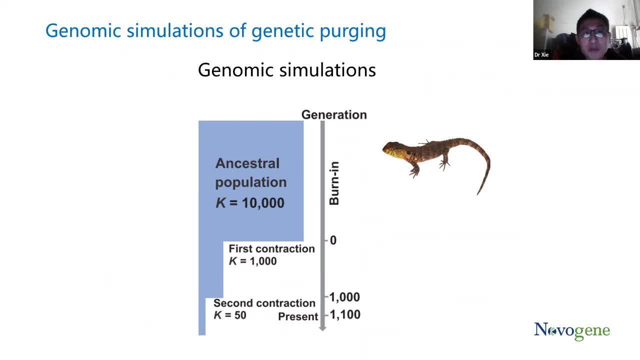 So we did some genomic simulations to confirm our results. This simulation is based on a model based on a demographic history of crocodile lizards. We modeled two population contractions of the crocodile lizards. One is about 1,000 years ago. it's about a dramatic contraction from an essential 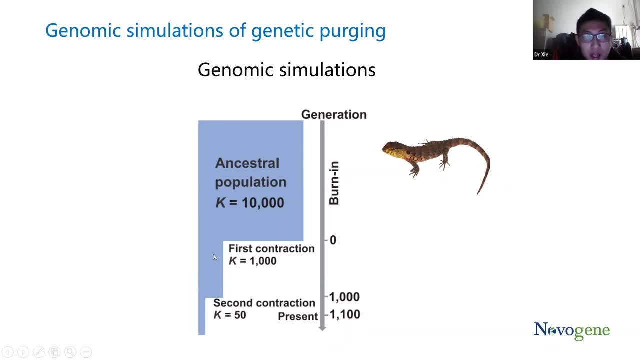 population size to about 1,000 individuals. And then another contraction, a second contraction about 100 years ago, which simulated the dramatic decline in recent years And from 1,000 individuals to about 50 individuals, this is to a very extreme small population size. 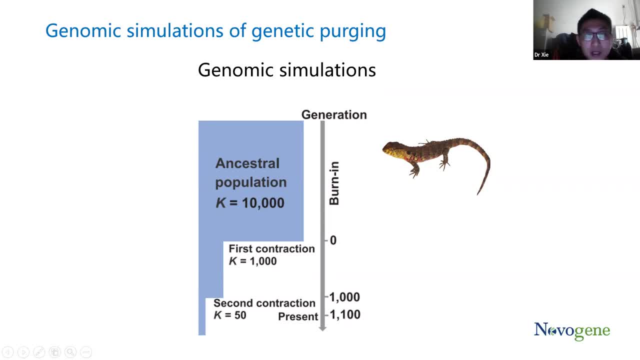 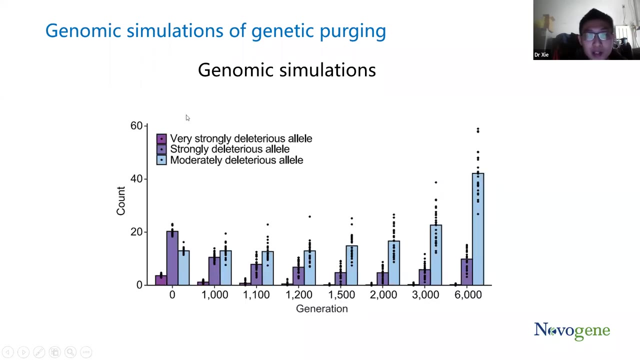 What we want to see in a simulated population, whether the deleterious alleles will be purged in this model And the results show that our simulation results are greatly confirmed with our empirical data, data, observed data of caudalisers, because 1,000 years is the end of the first contraction. 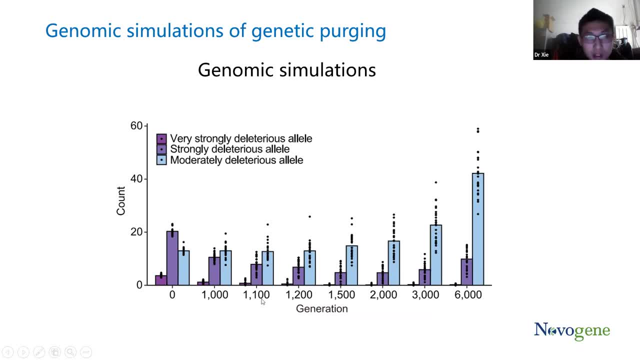 And 100 years following the second contraction, we can see that the very strongly and strongly deleterious alleles are all purged in this model, All purged in this short period of time. But for the moderately deleterious alleles, the purging- there's no trend of purging. 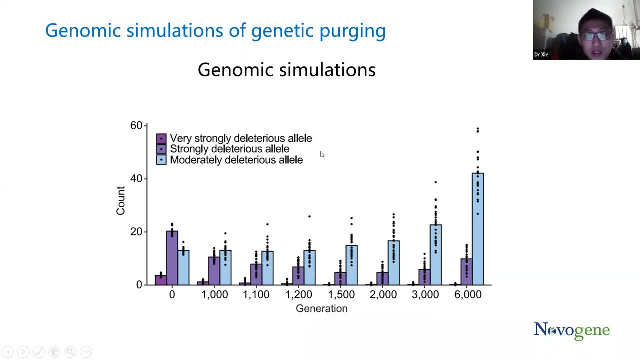 And in the long term we can see the purging of very strongly deleterious alleles continues. But for strongly deleterious and moderately deleterious, if the population stays in small population size for a fairly long time, we can see there's another trend. 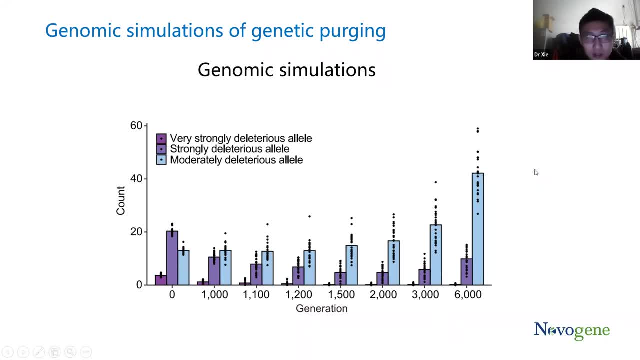 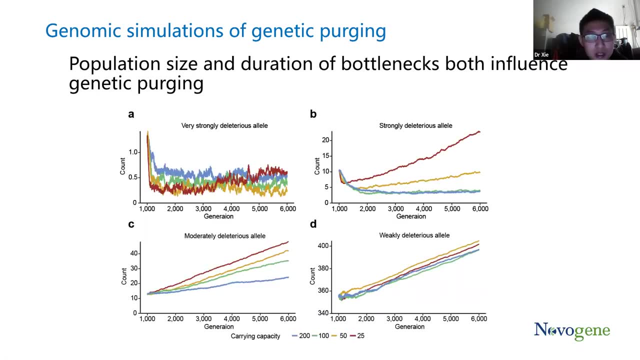 of decreasing for the deleterious alleles. We want to test whether this trend is persistent in different parameters. So we tried different carrying capacities, from about 200 individuals to 25 individuals. 25 is extremely small And we see there's a fairly consistent trend. 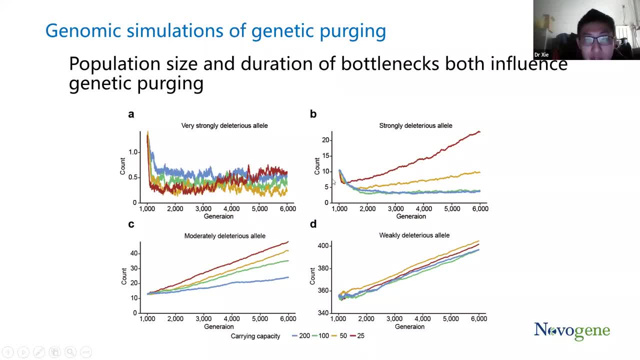 With the population size decreases, the purging effect enhances in the initial period. However, in the long term, when the population size is small, the overall the increasing of deleterious alleles become more severe in the long term. So we found that both the population size 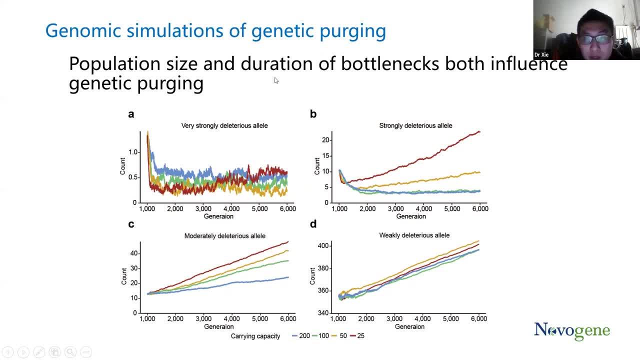 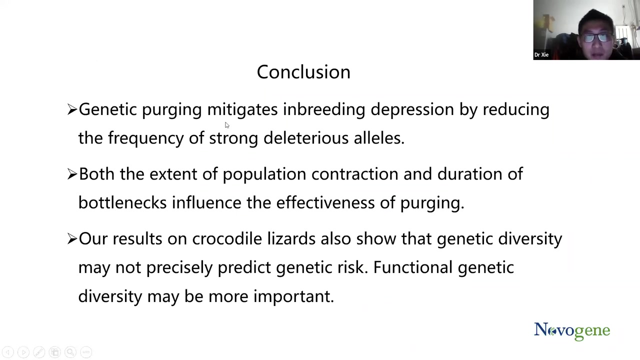 and duration of bottlenecks influences the process of genetic purging. Finally, from the results of our observed data and model results, we come to some conclusion. Firstly, we found that genetic purging mitigates the inbreeding depression by reducing the frequency. 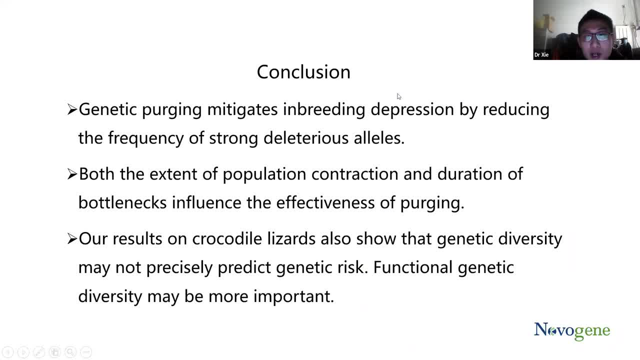 of strong deleterious alleles. This result comes from our observed data from crocodile lizard populations, as well as the model results. And second is that both the extent of population size and duration of deleterious alleles are very different. The duration of population contraction: 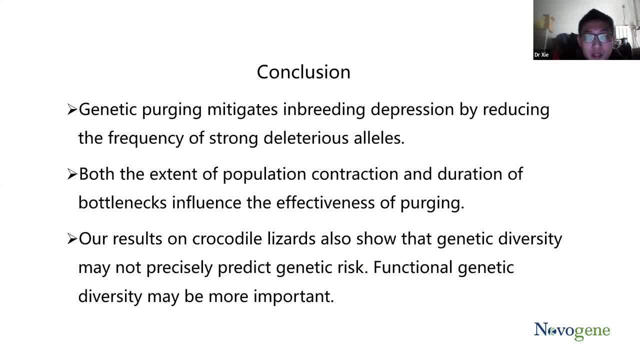 and the duration of bottlenecks influence the effectiveness of purging. This mainly comes from our simulation results. We found that when we reduce the population size of a second contraction, the purging become quicker, But in the long term the increasing trend. 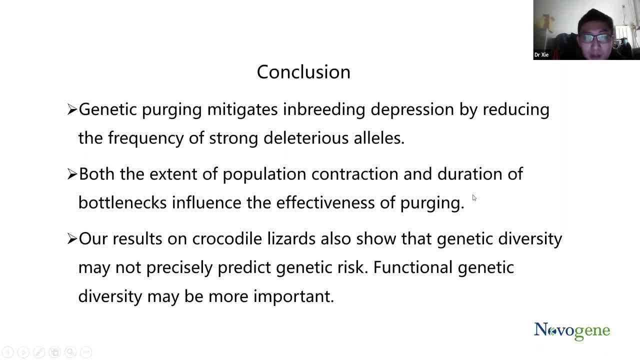 of deleterious alleles also become quicker for a small population size. We found that this is mainly because the decrease in genetic diversity and the fixation of some mutations contributed to the increase of deleterious alleles. And finally, our results show that on the crocodile lizards, 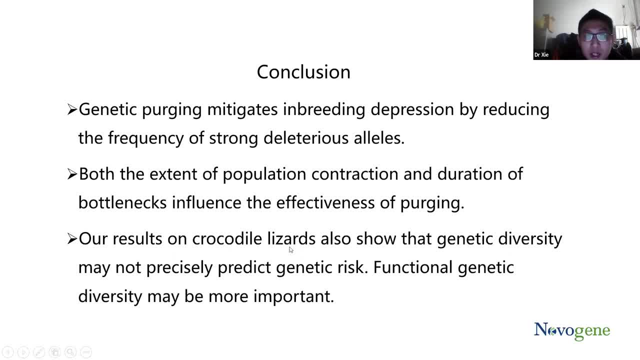 it has fairly low genetic diversity and high level of inbreeding, but the purging is working fairly good. So it shows that genetic diversity may not be precisely predict the genetic risk of crocodile lizards, And functional genetic diversity may be more important. 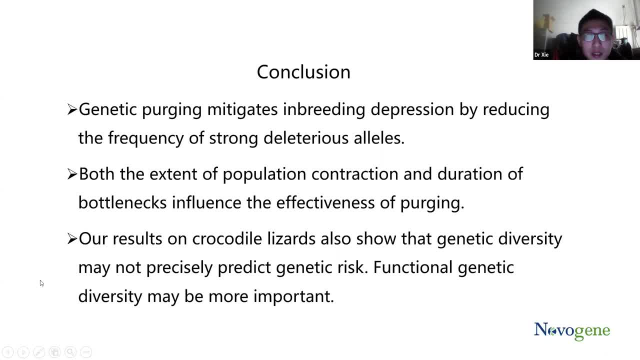 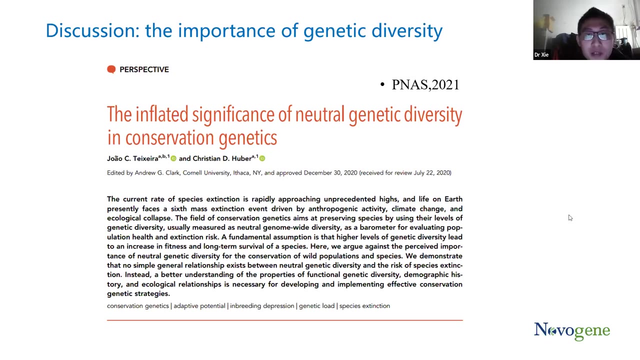 This one comes out from our discussion and some ongoing debate on the importance of genetic diversity, which we will discuss about later. The discussion about the importance of genetic diversity comes from a very perspective article published last year, Because the significance of genetic diversity has been studied for decades in conservation biology. 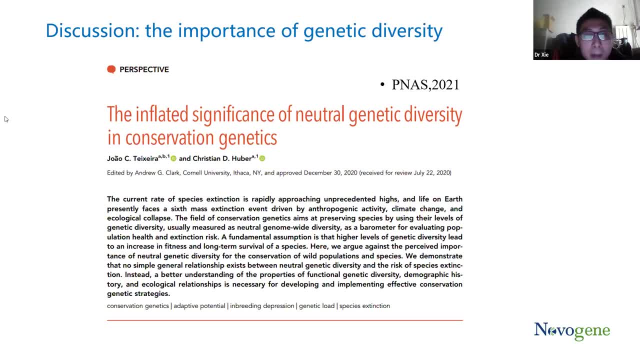 But last year a prosthetic in PNS. they argue that the infracted significance of neutral genetic diversity. the paper want to say that the genetic diversity will not precisely predict extinction risk of wild populations. So something about the functional diversity or the population history. 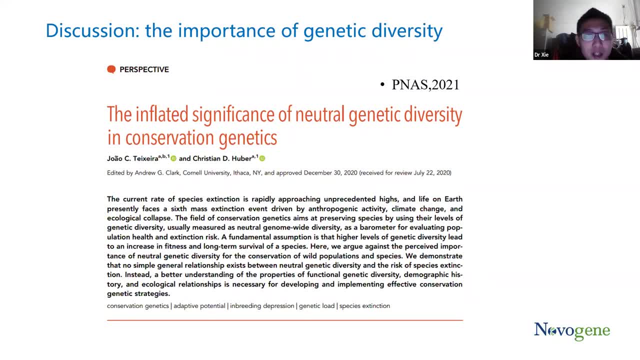 or the deleterious alleles will be more important. However, no student of this perspective article has been published. There's another article in publishing molecular ecology about several months after that. it argued with opinion. It says that the long standing significance of genetic diversity in conservation 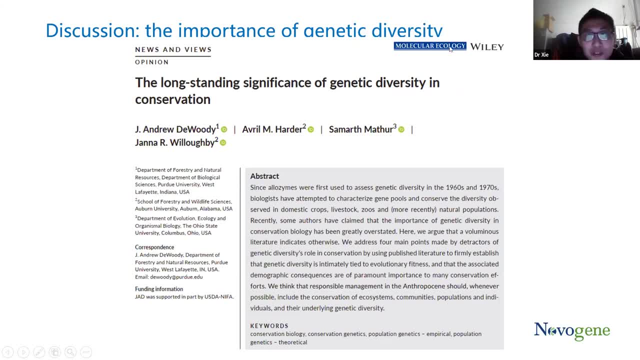 which listed our decades of research from all areas of conservation biology that support ideas. genetic diversity is very important in predicting the extinction risk of populations. And another more popular article it also published about November last year on PNAS. it again argued about the previous article that it says that genome-wide genetic variation 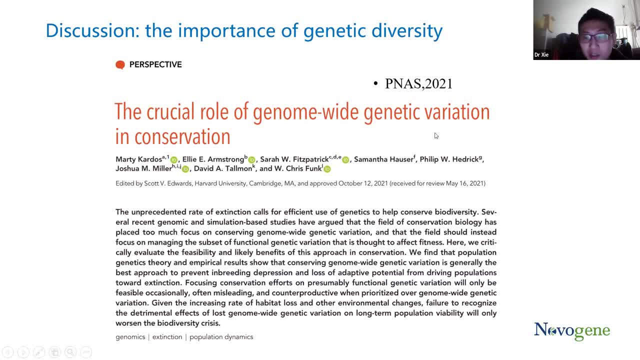 is very important in conservation. We know that the argument of these ideas is important, but the more important thing is some real data or evidences from case studies, And case studies actually is still emerging in recent years or months in recent time. For example, in PNAS last year, also in the fourth quarter, there is an article, the genomic. 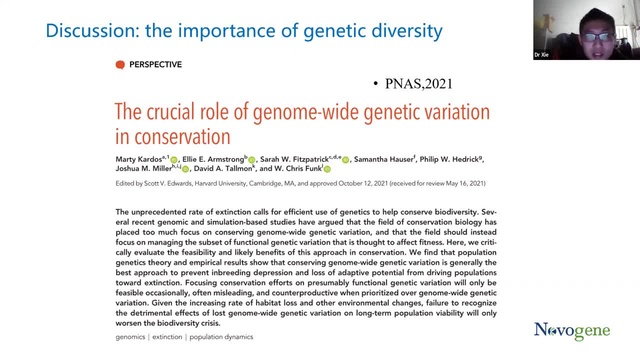 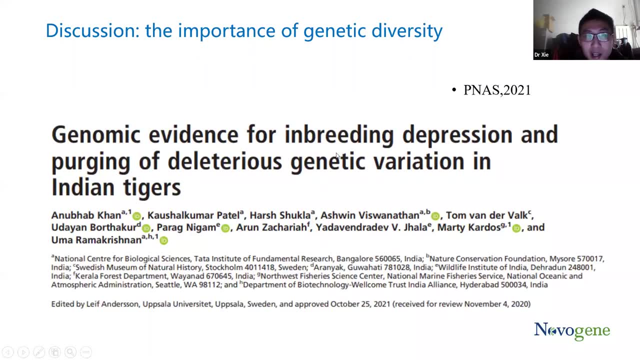 evidence, The genomic evidence for inbreeding, depression and purging of deleterious alleles in Indian tigers. They investigated genetic diversity and inbreeding and how deleterious alleles are purged in Indian tigers And it supports the idea that deleterious alleles can be greatly purged in Indian tigers. 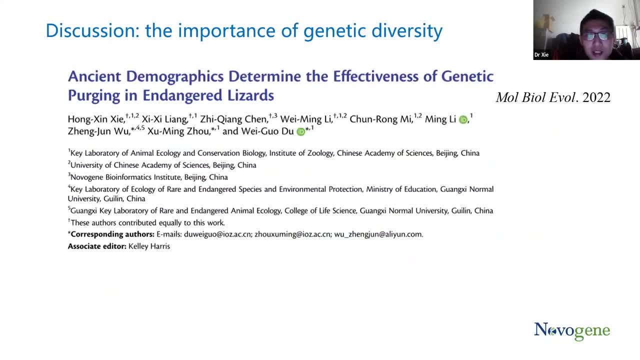 And another article is published recently. it's our work. we also- the data we provided and the simulation work We started- also support the idea that genetic purging are able to reduce inbreeding depression in the wild. So maybe genetic diversity may not be a good indicator, but we also found that population. 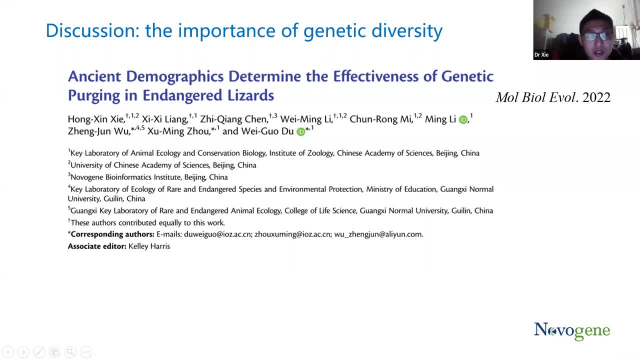 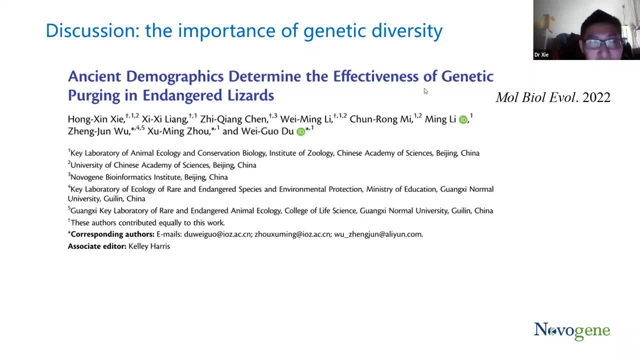 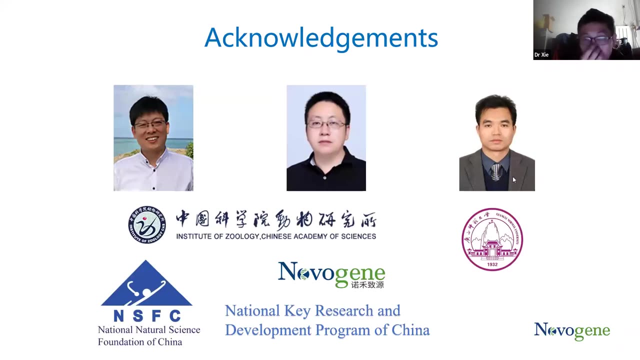 Thank you, Thank you, Thank you, And our work, our work. many thanks to Professor DeWei Guo and Professor Zhou Ximing. Our job is mainly under the guidance of these two professors, And Professor Wu Zheng Jun provided important samples from the crocodile lasers. 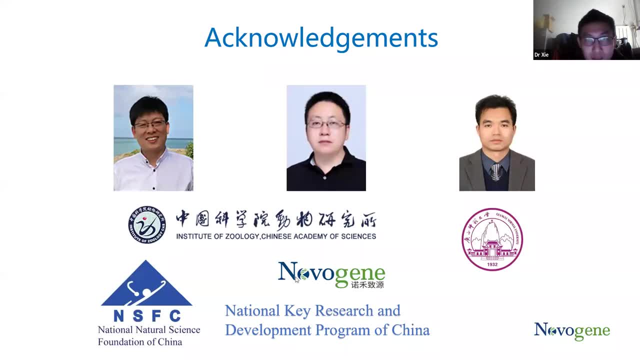 And also for all, many thanks to all the authors from our lab And thank you, Thank you, Thank you. And this job is funded by National Natural Science Foundation of China and National Key Research and Development Program of China. I may be talking a bit quick, so if there's any questions, please freely ask any questions. 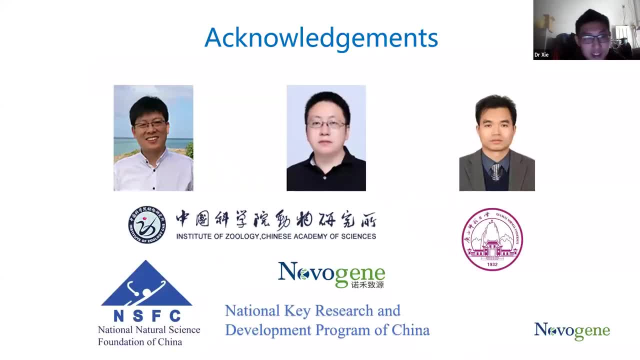 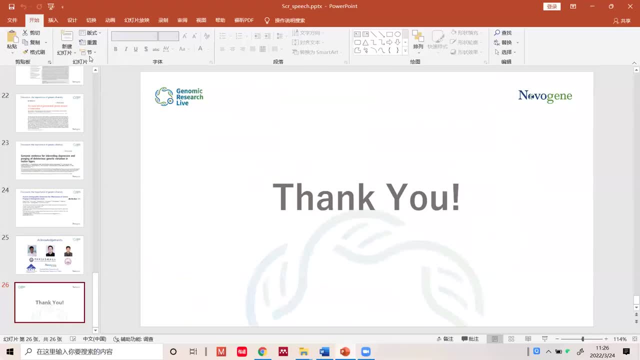 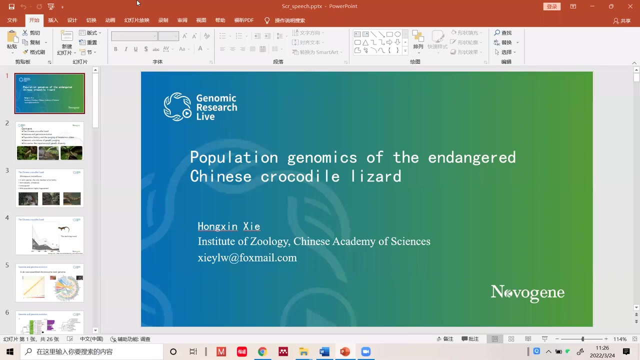 I'm very pleased to answer. Thank you so much for this comprehensive and in-depth lecture, And now we will take a few questions from the audiences, And the first one is from an anonymous audience, that what strategies are generally adopted when sampling wild crocodile lizards and their methods to assess the representativeness of the samples. 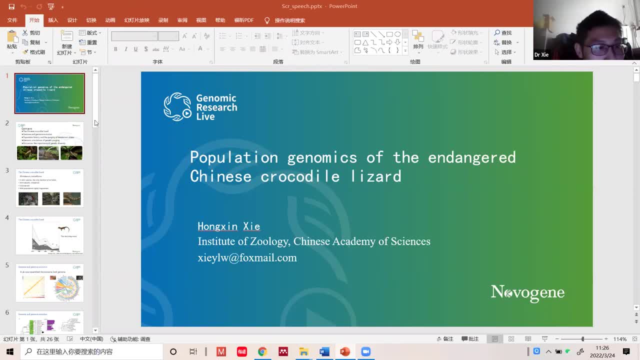 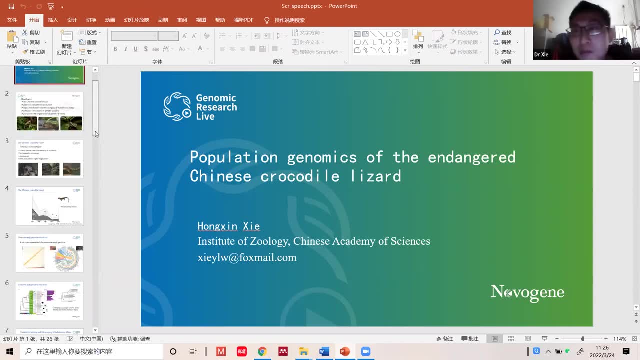 Well, I talk about it a bit in my presentation, but I will discuss more, because in a case like this, in a case of sampling endangered species, the problem is that, because it's endangered and the population size is small, there's very like chance that we sampled two very close related samples. 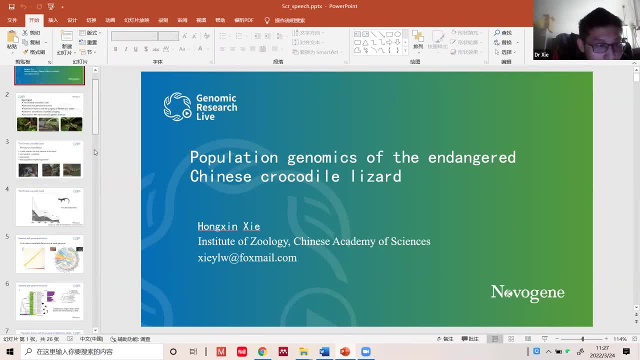 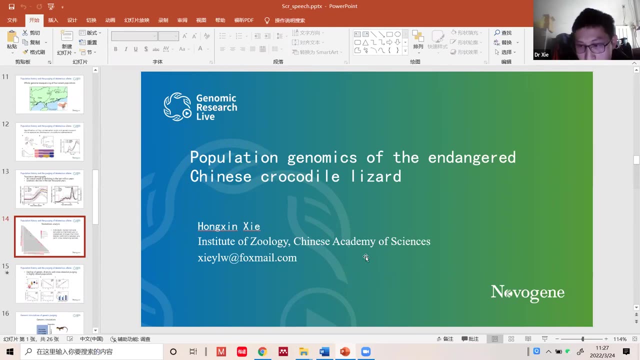 So the first step is that we try not to sample the same individuals in the same place, That's in the sampling procedure, But second in the data analysis, data analysis: when we are doing the data analysis, it's very important to do a readiness analysis. 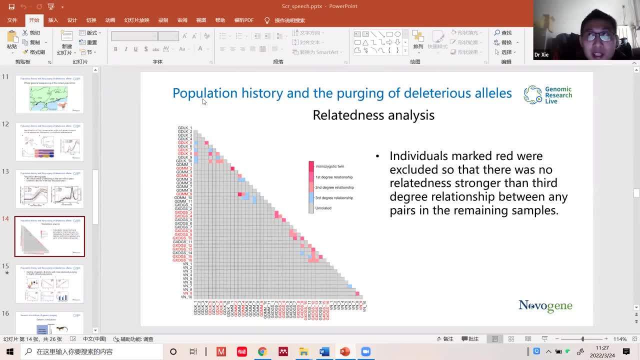 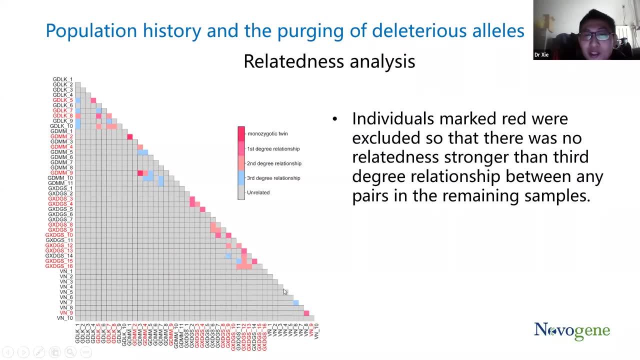 This analysis. if you did not do it, maybe in the article review process reviewers will ask you if you did a readiness analysis. This may not influence your results very greatly, but doing it is necessary because it will reduce some biases from your analysis. 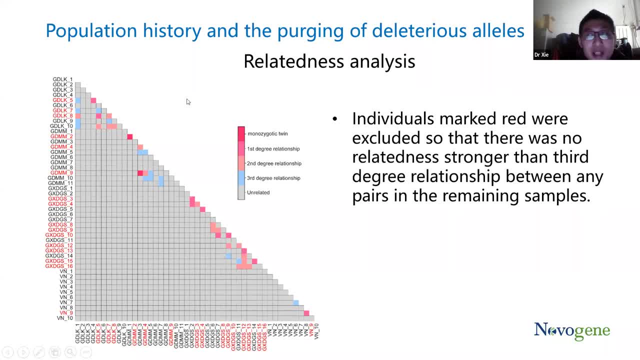 So in doing so, we excluded many individuals that are possibly close related, And actually, in our case, the amount of individuals that are possibly related is actually large. But it's good. You should remove all individuals that are possibly close related. So, after this analysis, 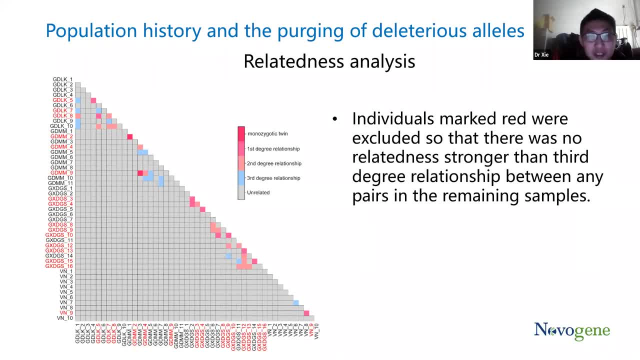 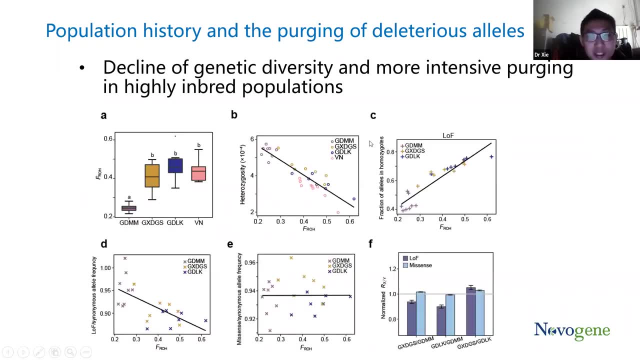 the another. the statistical significance actually did not change a lot because we showed a more clear trend in our Fourier analysis, the many in this part. We did two parts. We did two analysis, actually The first one we did not do the. 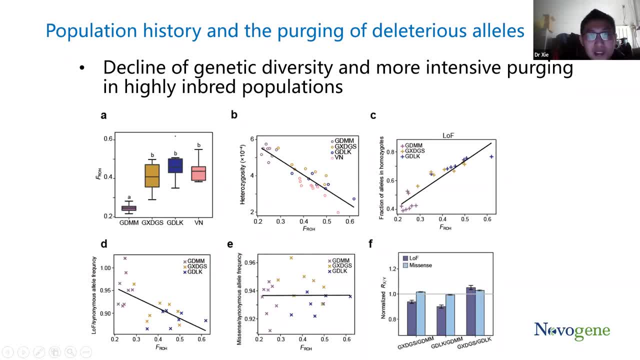 we did not do the readiness analysis, But in the final version we did. we excluded all the samples And we found that the overall trend is more clear when we excluded all the samples. So I think we did a good job And also 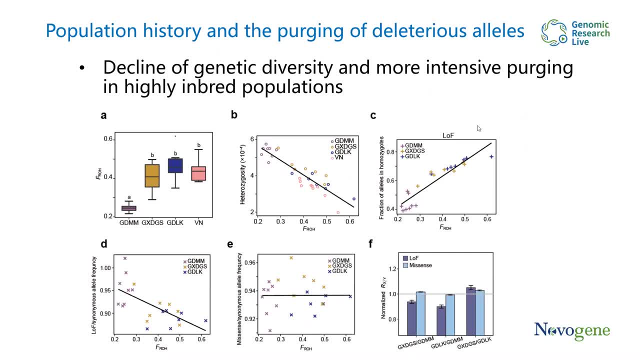 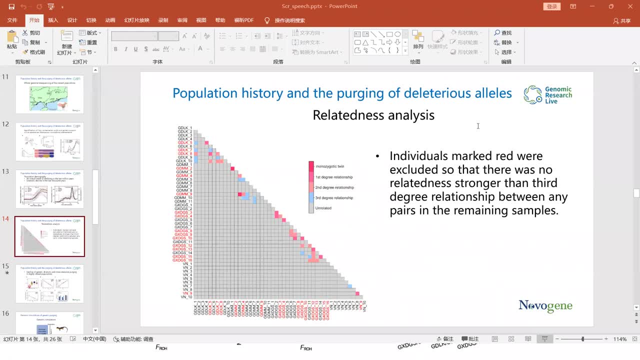 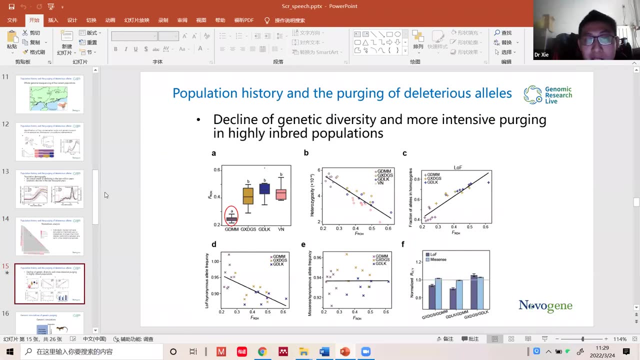 thank you, and the second question is from Lou. The PopSize ABC can also predict millions of years of population history And how to choose between the softwares to predict the population size? Currently there are many different softwares in solving population demography. 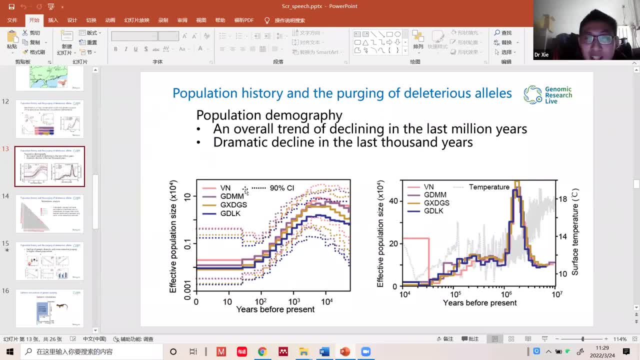 And the popular one is PopSize ABC, one is PSMC and there's also MSMC and other methods. And we choose these two methods because we want to solve the history- The most important history is the most recent one- because we want to 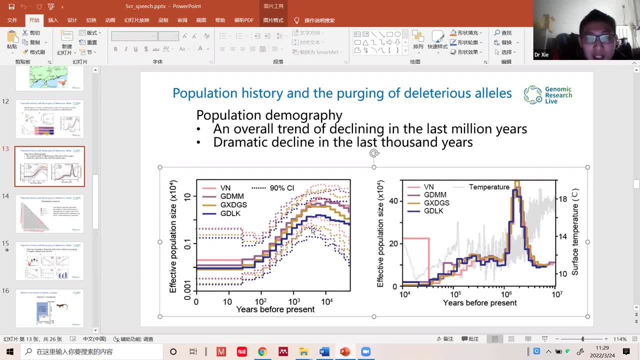 see where the population size is decreasing in crocodile lizards. So we chose to use the population size ABC. This method is more precisely predicting the more recent histories, mainly from 20,000 years to present. But the PSMC is accurate and popular. but this method can only. 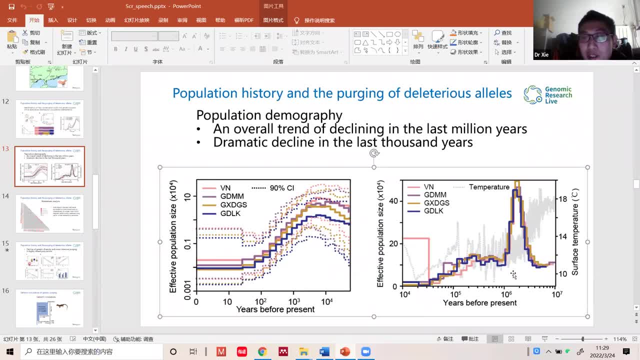 solve the histories more ancient than 20,000 years ago, But in a more recent history. it is not precisely. it was not precisely predicted, And it is. this is illustrated in his original article. So in our, in our study, we choose to combine these two methods. 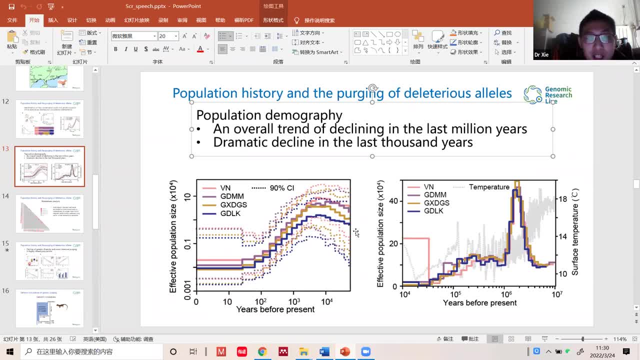 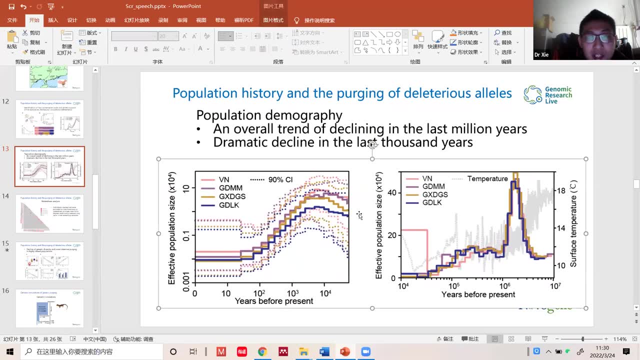 in order to solve the history of crocodile lizards. So we choose to combine these two methods to have a more broad view of the population history of crocodile lizards And maybe, if there are more precise methods ongoing, if there's ongoing in the literature. 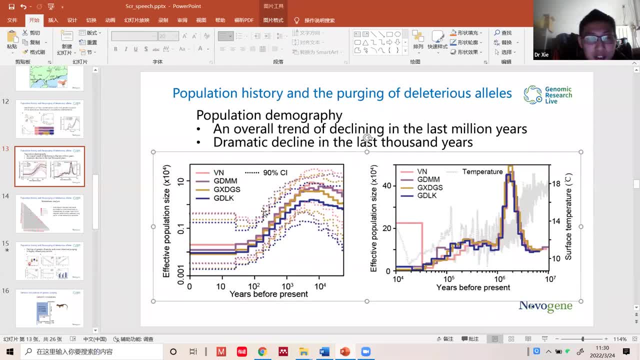 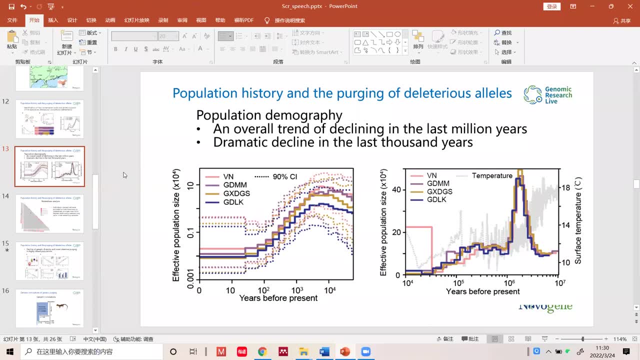 and when doing a research, you should choose the most proper one to your focal species. Great Thank you, Dr Xie. And the last question we have from the audience is that why there was a significant reduction during the population history? It is because there is. 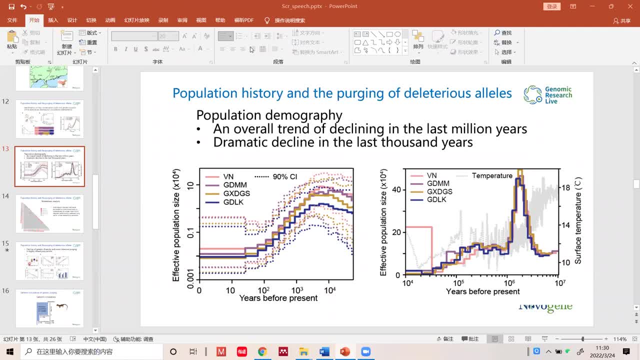 any climate change which can lead the situation, or is there any methods could be used to study the historical data? Is there any method used to study Our reconstruction of population history? mainly comes from our re-sequencing data, which is the data that we use to study the population history. 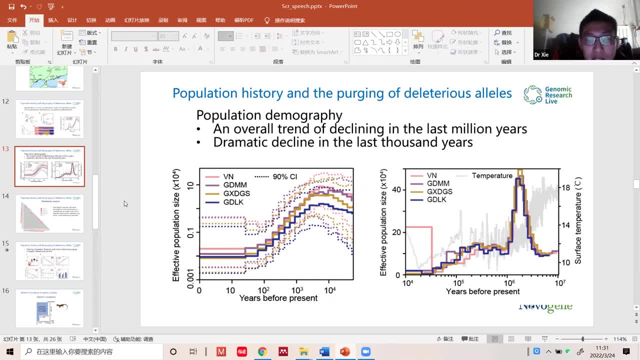 The re-sequencing data is the DNA data, genome data. We just estimated from our current data the overall trend in the history. But actually there may be some real data that will describe the trend in history, Maybe some data from fossil records Or there's another way of predicting. 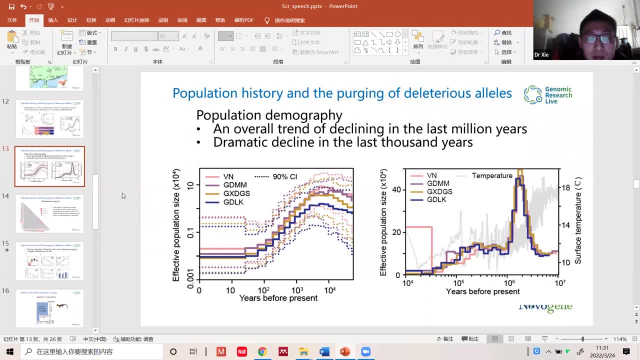 the distribution, the SDM models, species distribution models. We actually also did that, the species distribution models, who describe the possible distribution of a species in the past, And we did that actually but not presented in our final paper. We found that the species 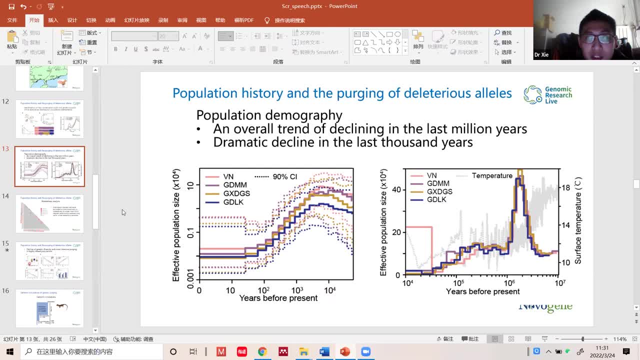 distribution model in the current situation for crocodile lizards is actually far broader than its actual distribution, which shows that actually there's many suitable habitats around, but the real population size is small. So we have to look at the distribution model in the current situation. 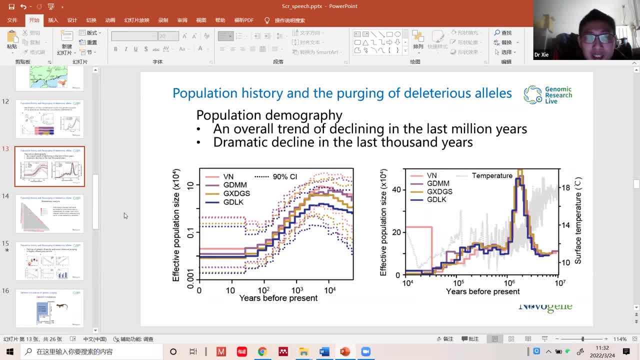 It shows that maybe human activity is a human activity that drives the extinction of this species, but not its natural adaptation to the environment, And in many cases it's very popular to use both the SDM models and the sequence and the demographic estimation from genome data to 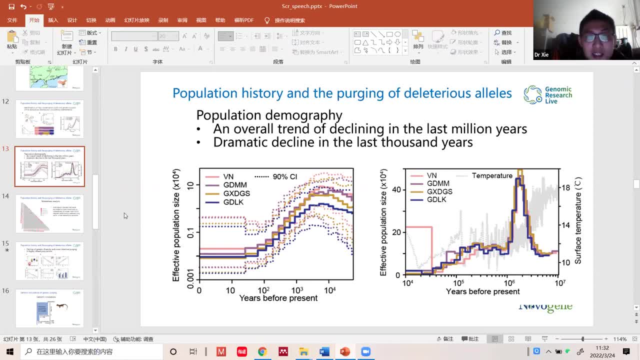 combine these two data to analysis the man-driven of extinction of the species, And there may be many literature using combining the two methods, But in our current work we did not put the SDM model because we just want to know that the population is declining. This is a very important information.